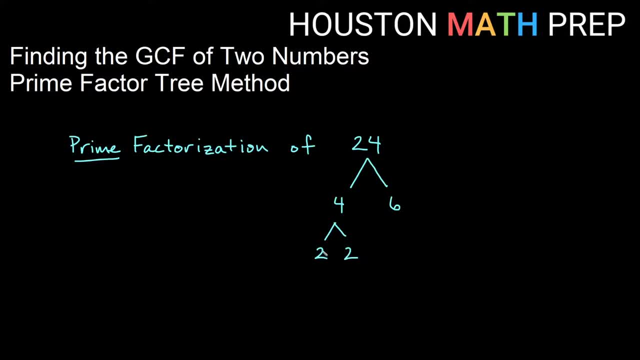 Now, 2 is a prime number because it is only 1 times 2, as far as factors go. So both of these are prime numbers. I'm going to circle these on my factor tree And then with 6. also, 6 can be broken down further into. 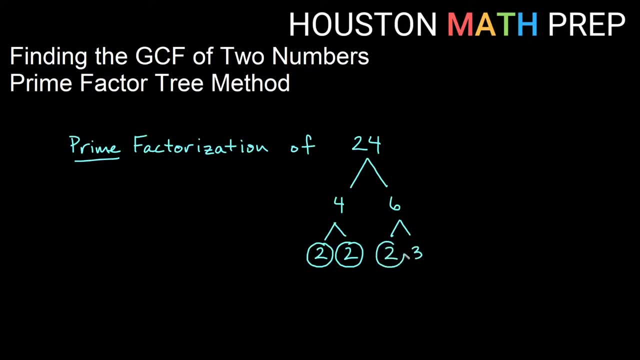 2 times 3.. So we have prime factors of 6 being 2 and 3.. So if you look at everything that is circled in my factor tree that tells me that 24, the prime factorization of that is going to be 2 times 2 times 2 times 3.. 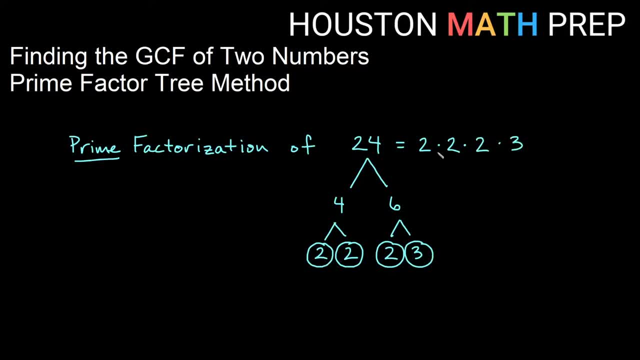 I'm going to write them in ascending order, so lowest first up to highest. So we have 3 copies of 2 and 1 copy of 3.. That's the prime factorization of 24.. Let's do one more And let's do it with 60. So prime factorization of 60 may. 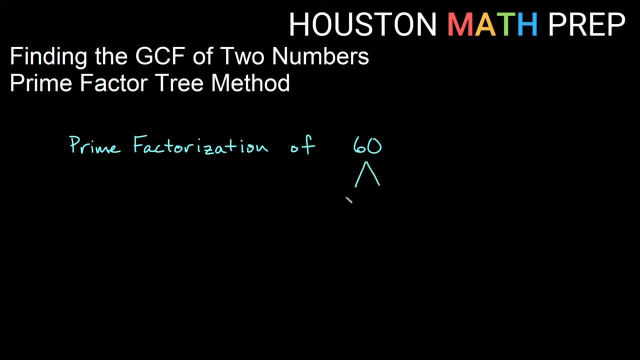 be an easy thing to see. That 60 is would be 6 times 10.. So in this one we know that 6 already breaks down into 2 times 3.. So we'll keep breaking it down until we get to there, And those are both prime numbers. 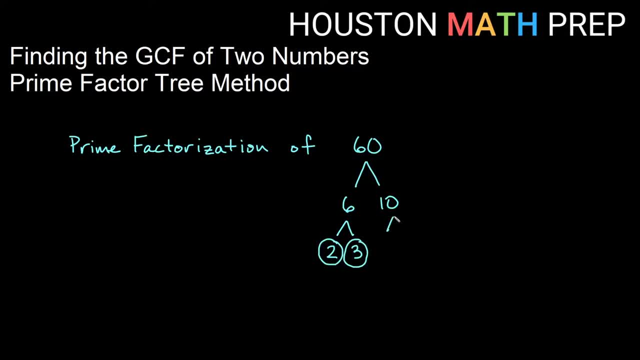 So we'll stop with those And then with 10,. I can break 10 down further into 2 times 5.. 5, and those are both prime numbers. Neither of those can be broken down further except to 1 and themselves. So if I write these in ascending order, write the smallest one first. 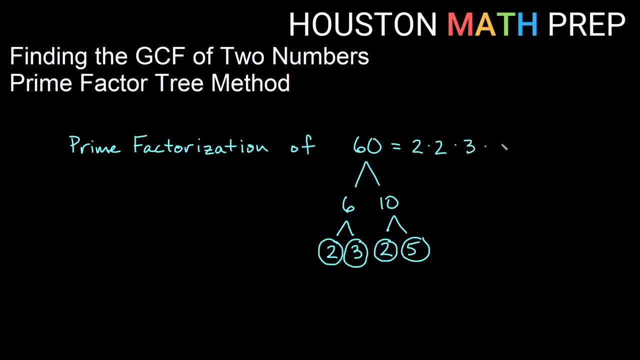 that would give me 2 times 2 times 3 times 5, and that's the prime factorization of 60.. So I've just written these in ascending order. Okay, looking at these, you can see if we're trying to find the greatest common factor of 24 and 60,. what we will do is we'll go. 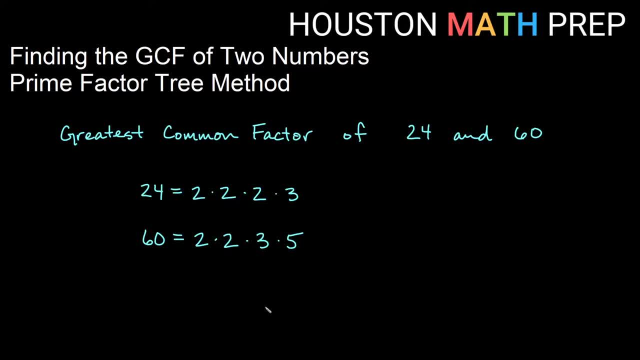 through each factor on the list that we have in both, and then we will pick out however many they have in common of each factor. So the first thing I see is there are 2s on each list. So since there are 2s on each list, I say: how many do they have in common? This: 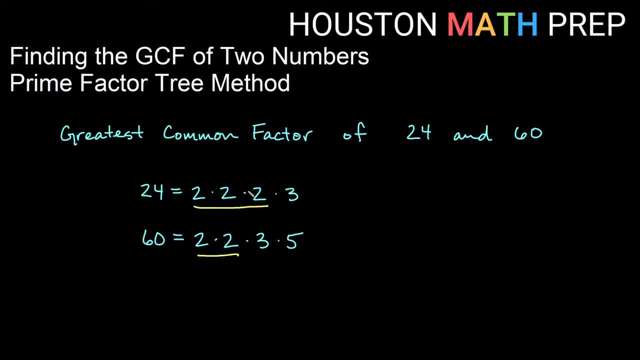 one has 3 copies of 2, this one has 2 copies of 2.. They don't both have 3 copies of 2, so I can't use 3 copies of 2.. They do both have at least 2 copies of 2.. Okay, so that. 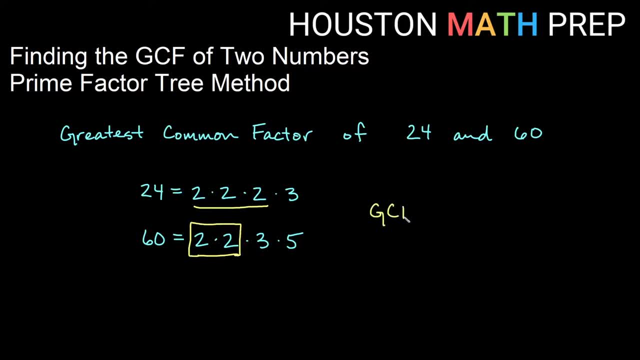 tells us that we have 2 copies of 2, and that tells us that we have 2 copies of 2, and that tells me that the greatest common factor is going to have 2 copies of 2 as part of its prime factorization. Then the next thing I look at: they both have 3s and they both. 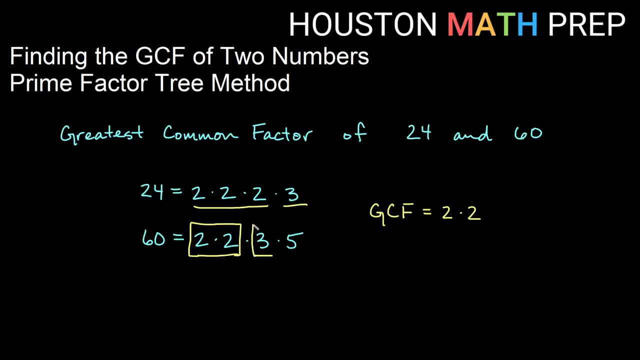 have 1 copy of 3, right? So they both have at least 1 copy of 3, so I'll go ahead and put a 3 in there as well. If I look at, 60 has a prime factor of 5 in its factorization. 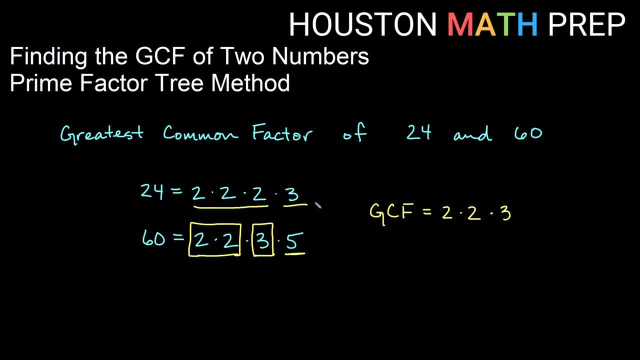 but there is no factor of 5.. So since they do not have a 5 in common, both of them, 5 isn't going into both of them. then I wouldn't write that down. So my greatest common factor, the prime factorization of 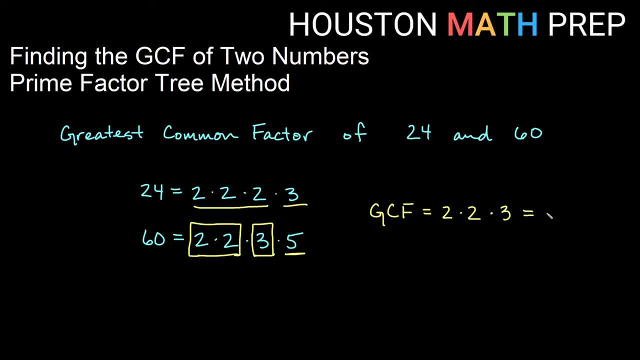 that is going to be 2 times 2 times 3, which would give us 12 as the greatest common factor. Now some of you might be able to look at 24 and 60 and already see what goes into them. You might see all the factors and you might even be able to see that 12 is the greatest. 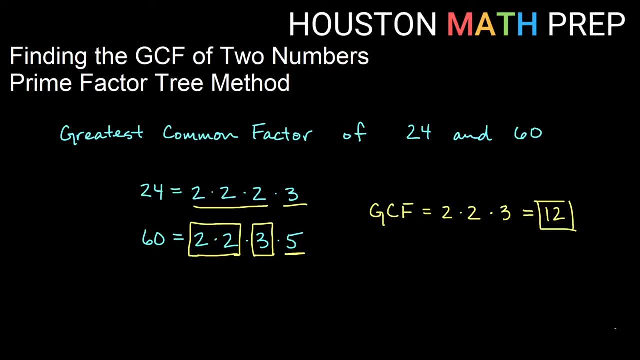 common factor, and that's great. What we want to be able to do is use this type of factor, this type of thing, if the numbers don't have much in common or they're much larger than we're used to dealing with and we're trying to figure out what it might be. 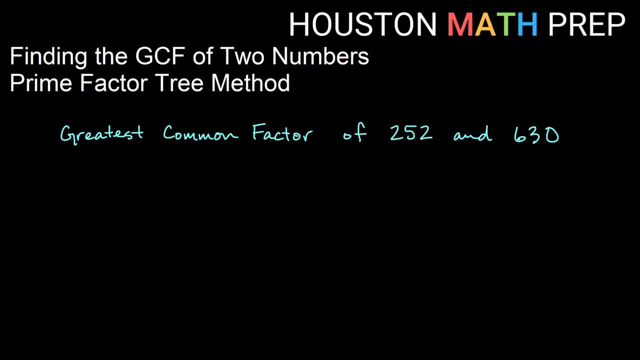 Let's look at another example here. So if we have the prime factorization of 252 and 630.. So let's first look at 252.. It ends in an even number. so I know that it's divisible by 2. So if I cut it in half I would say it's 2 times something right? So 2 times. 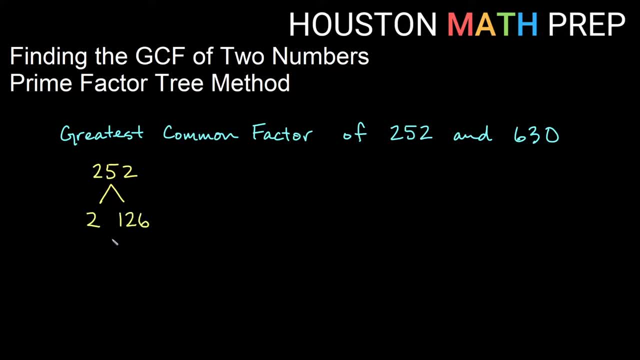 divide that by 2, it'll give you 126.. Now I know that 2 is a prime number, so I'm going to keep that. 126 is still an even number. it ends in 6, so I know that I can at least. 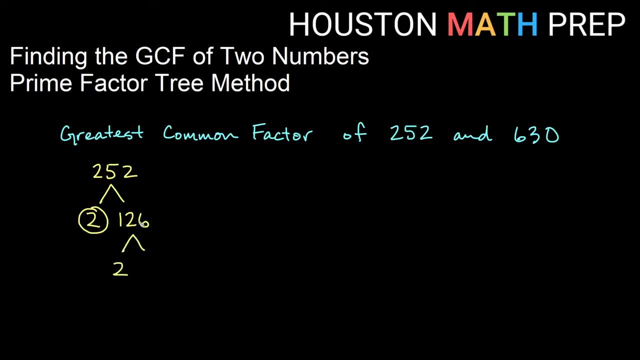 break that down into 2 times something else, right? So 2 times something gives me 126.. If I'm not sure, I can take 126 and divide by the 2, and that will give me 63. So I break. 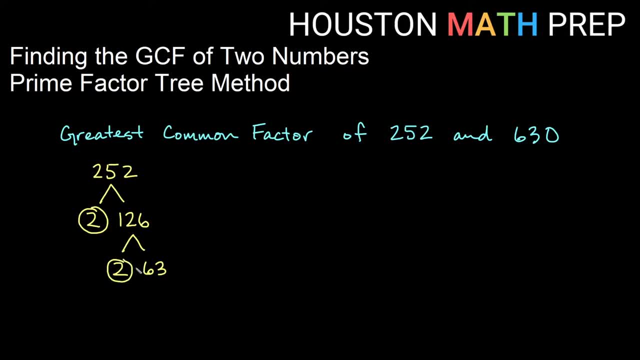 it down into 2 times 63. And again, any order that you see the factors in and you break it down, you'll get the same thing in the end. So 63, I could break down as 9 times 7.. 9 can be broken down further, 7 cannot. so we'll. 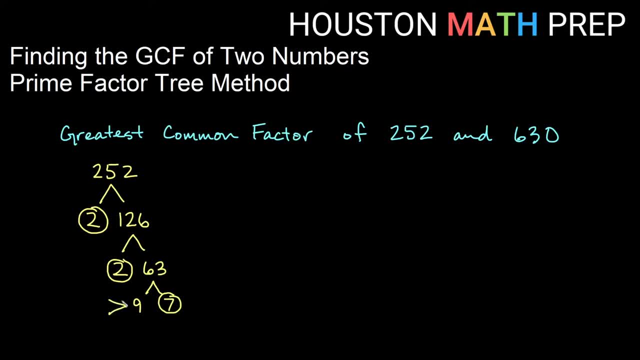 keep the 7. And then the 9,. we'll go ahead and we ran out of room here, so we'll go ahead and say 3 times 3 for the 9, and both of those 3s are prime. So if I write the prime, factorization. 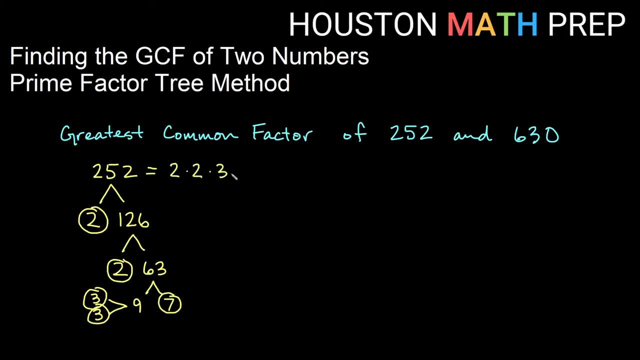 for this. that's a pair of 2s, a pair of 3s and a 7.. So let's do the prime factorization of 630.. So if you, you know, maybe you see that it's divisible by something, I'll just 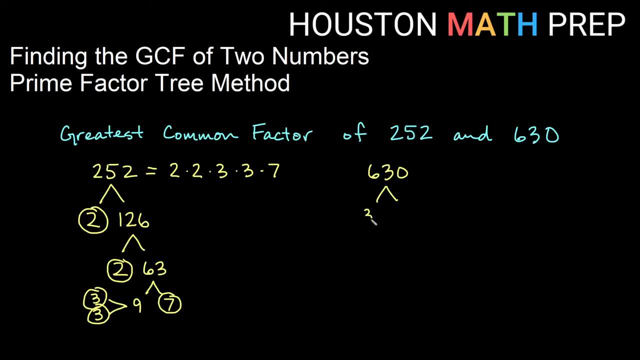 say: I see that it's divisible by 3, let's say So. I say 3 times, something will give me 630.. So 630 divided by 3 is 210.. 3 is prime, 210 is not. So let's say I break down 210,. 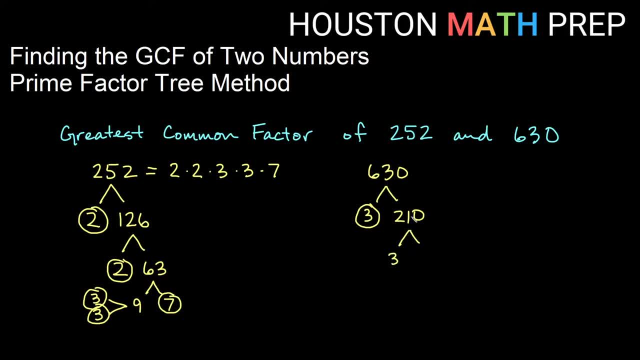 and I could say it's maybe. it's divisible by 3 again. So 210 divided by 3 would give me 70. So 3 times 70. The 3 again is prime, the 70 is not. So if we break it down further I would have maybe. 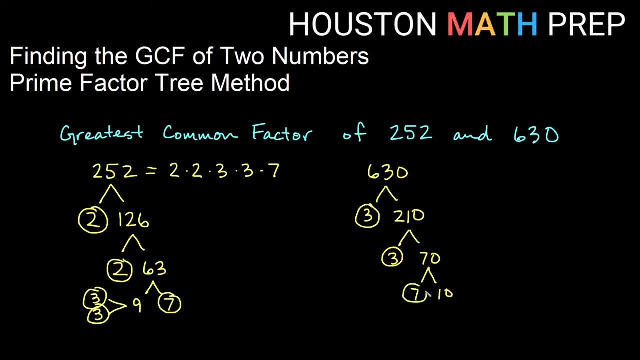 like 7 times 10.. The 7 is prime here, and then the 10 will break down into 2 times 5, and both of those are prime as well. So we get that the prime factorization of 630 is going to be one copy of 2. there I have a pair of 3s, I have a 5 and a 7.. So if I write 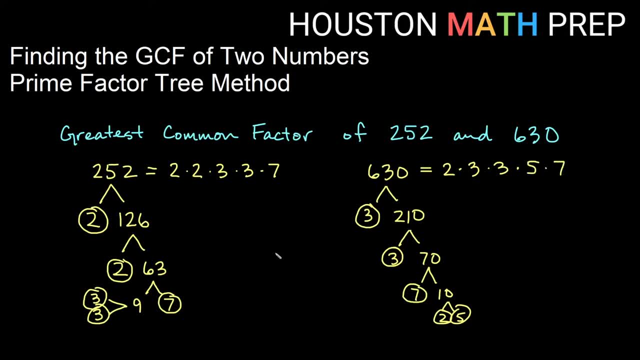 all of that down, I get that as the prime factorization. And now if I look at what is in common and how many are in common, So here I have two copies of 2.. Here I have only one copy of 2.. So we have one copy of 2 for sure in common. 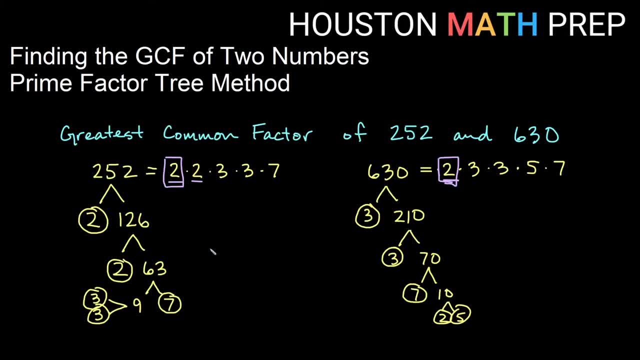 So I will keep one copy of 2.. So the greatest common factor will have 2 in its prime factorization. If I look at the 3s, both of them have a pair of 3s, So they share a pair of 3s and they 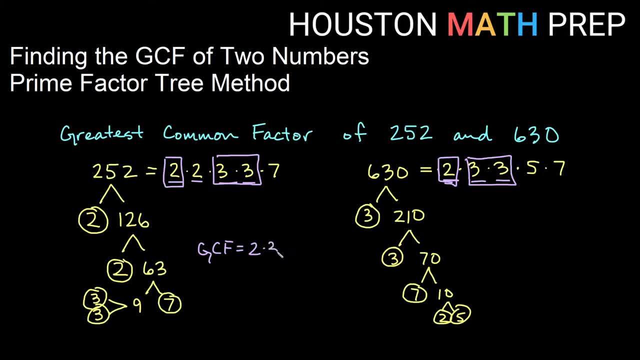 share a pair of 3s in common in the prime factorization, So I will also write down a pair of 3s. You notice this one over here- 630,, contains a 5.. This one does not contain a 5,, so they don't have a 5 in common. They do, however, have a 7 in common. They both